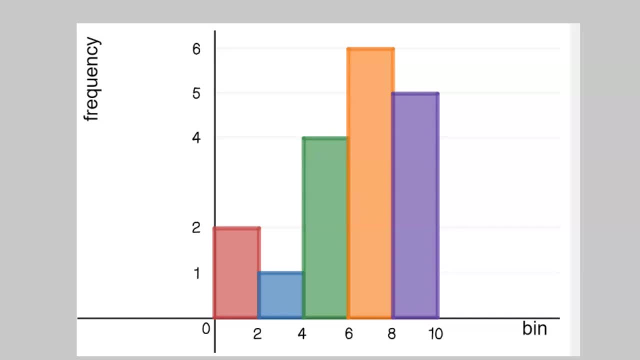 Can be trickier with the histogram, So I've just grabbed this histogram offline, which is bad on my part, but I didn't want to come up with one. So you can see here in this histogram it looks like we have- I just want to make sure my pen isn't too big- two, three, seven, 13,, 18 values in this particular data set. I don't know why they colored the different bars, but whatever We can see there's two, one, four, six and five. 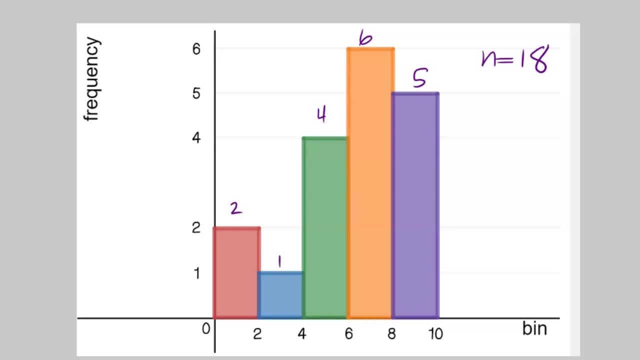 Uh, values in these particular bars. So you could still do the very basic counting in method of finding a median that a lot of people learn in like middle school, by just kind of dividing up these bars and then counting inward. So we'd want to start with the lowest value and make sure that we cross off a high value, so forth, so on, until we reach the middle. Now I gave you a histogram of 175 observations, So this is not reasonable to do. 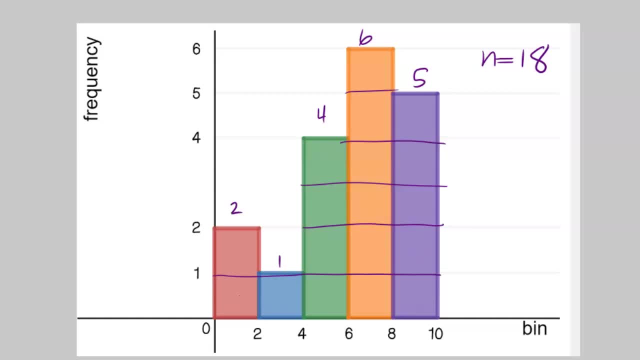 So what you're going to do instead on something where there's a much larger sample size, is you're going to want to go ahead and use that N plus one over two, that that location of your histogram, as a way to figure this out? Alternatively, you could just say: where is the 50th percentile right? Where's half of 18? Half of 18 is at nine. So I'd be looking at around the ninth observation. For this particular one, we have 18 plus one over two. We would actually be averaging the ninth observation. 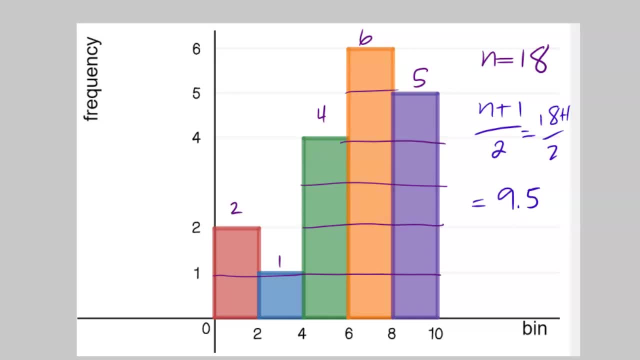 So we would be averaging the ninth and 10th observations because we'd end up right between them. So we're going to hope here that I don't have any problems. So now we could just count over to figure out where the ninth and 10th thing were: One, two, three, four, five, six, seven, eight, nine and 10.. So we don't know exactly what the value of the ninth or 10th observation is, but we do know that, whatever it is, it's between the value six and eight, not including eight. right.